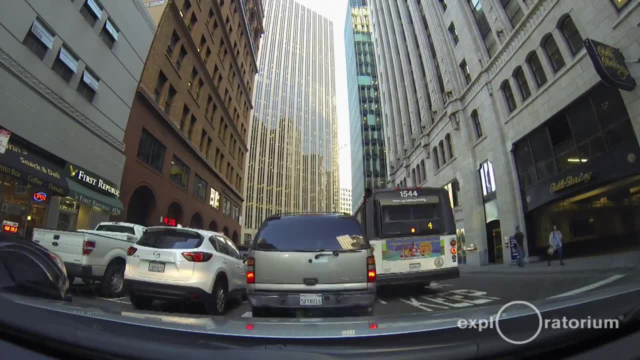 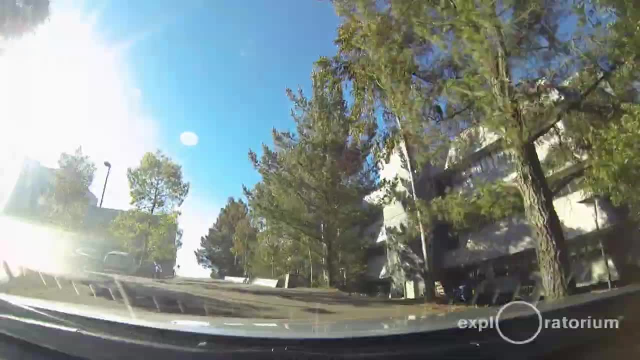 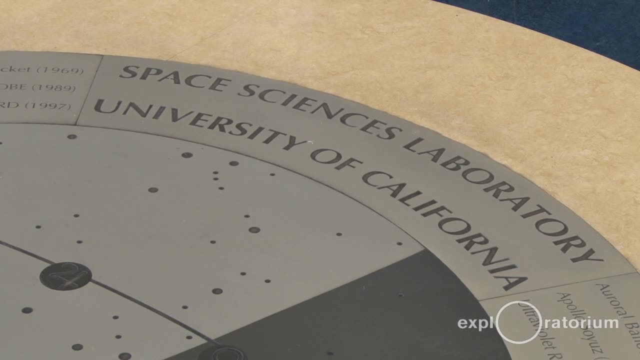 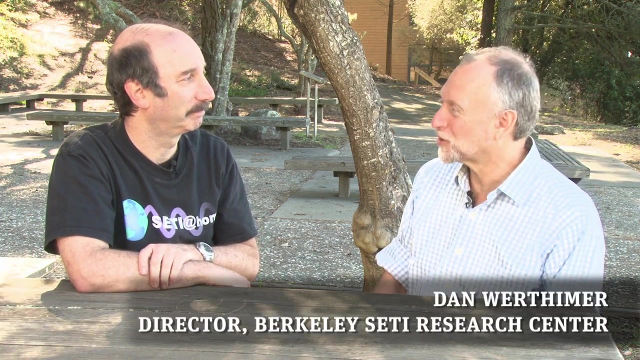 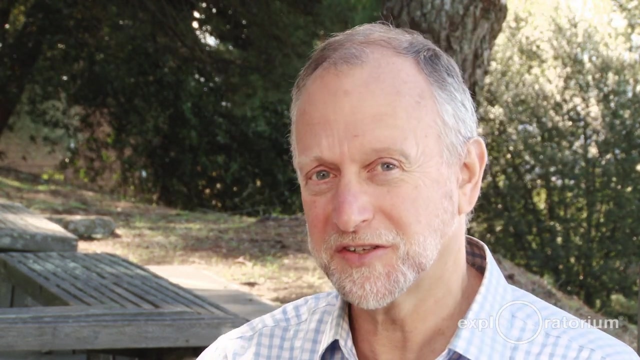 Dan, you're in charge of the SETI program here at Berkeley. Can you tell us a little bit about what SETI is? SETI is the Search for Extraterrestrial Intelligence. We're trying to answer the question: are we alone, Is anybody out there? And one of the ideas is that earthlings are sending off all. 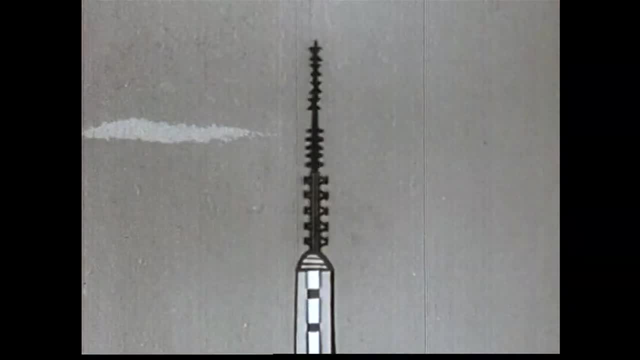 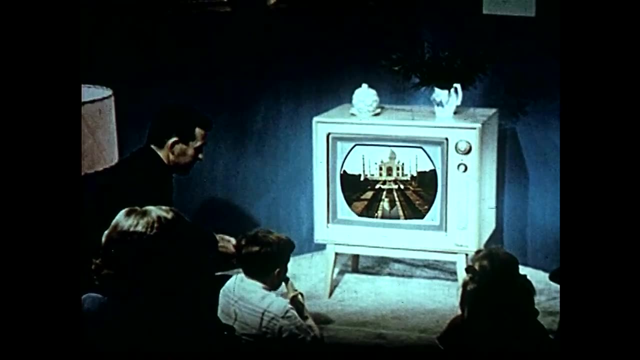 this radio and television and radar signals out into space unintentionally. like I Love Lucy, Ed Sullivan, have left the earth 50 years ago, have gone past 10,000 stars. the nearby stars have seen The Simpsons. So if we're polluting space with radio and television, 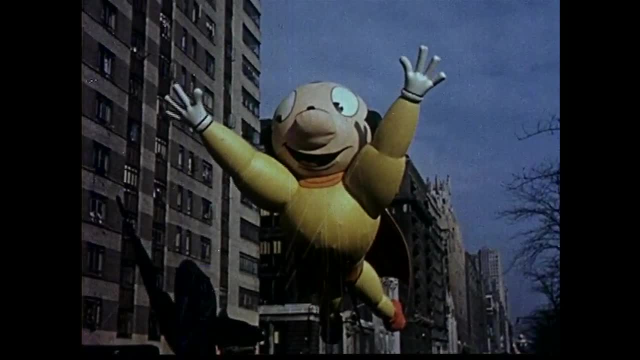 maybe other civilizations if they're out there, maybe they have something like that that we could detect. And that's what we're trying to do in SETI: and see if there are any of these signals out there and see if we're alone. 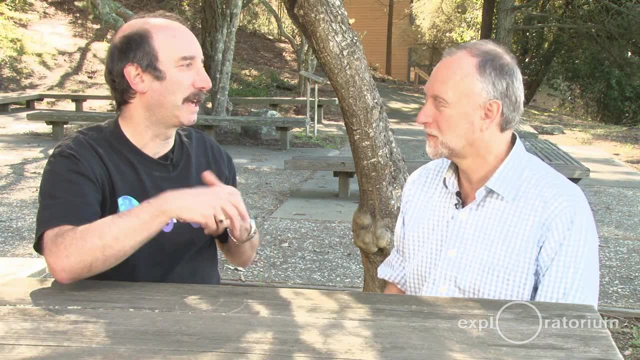 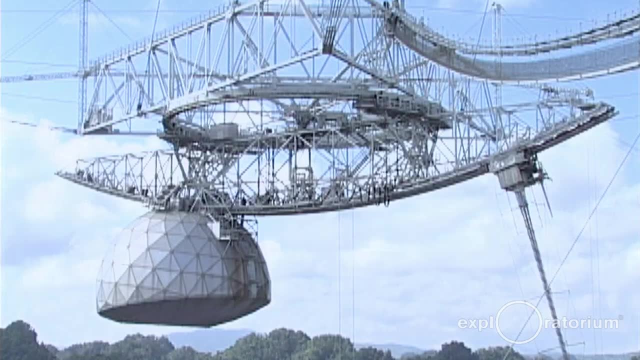 So it's not just, we're not just sticking an aerial up on our roof here. How do you actually detect it? The signals are likely to be extremely weak, So you can't find them with a little tiny antenna. So we use the world's largest antenna. We call it a radio telescope. It's the Arecibo. 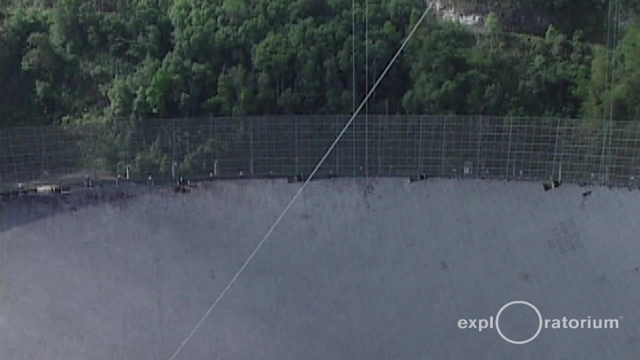 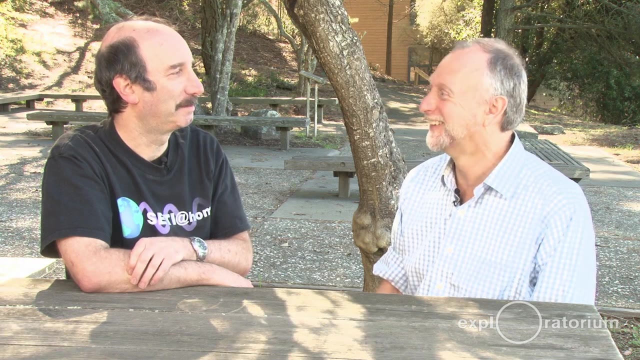 radio telescope in Puerto Rico. It's 1,000 feet in diameter. It would hold 10 billion bowls of corn flakes. We haven't actually done that yet, but we've made that calculation. You've put in an NSF grant for that. 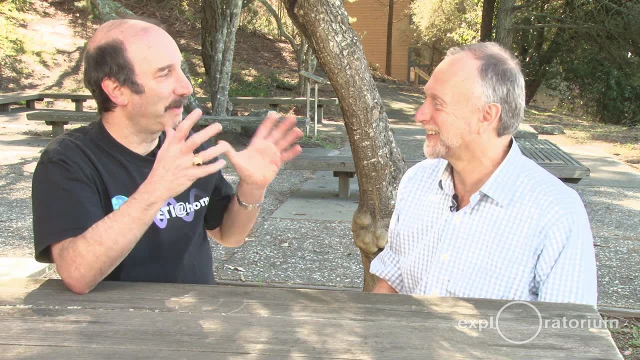 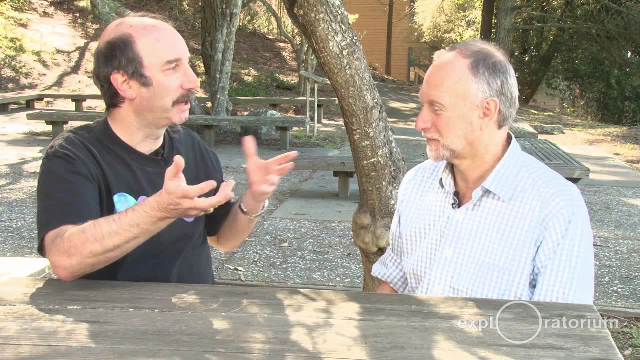 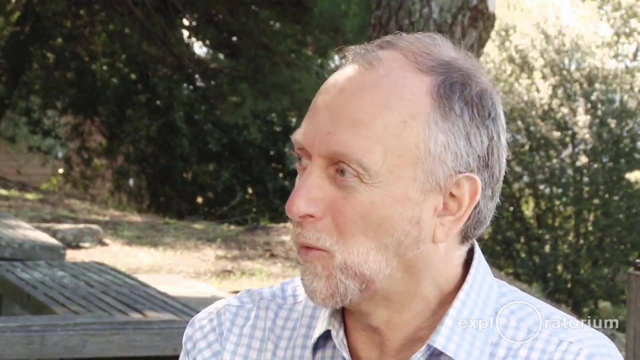 We should try that experiment. And so you receive them there and then now you have a recording of all these radio signals coming from space. How do you tell the difference between ET and all the other things that are out there? We need a lot of computing power to figure out where the signal might be. We don't know. 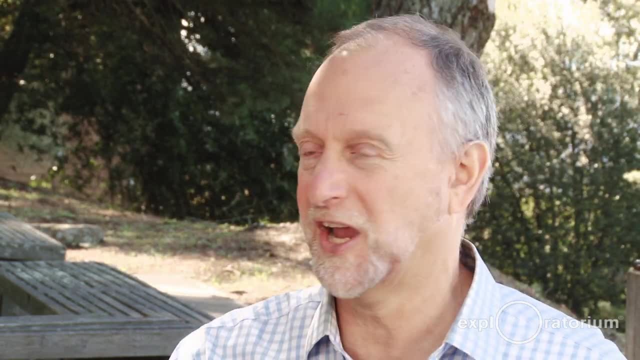 what frequency it might be at. so we have to listen to a lot of different frequencies, a lot of different channels. We don't know where to point the telescope, where ET might be lurking, so we want to point at all these different places in the sky. We don't know. 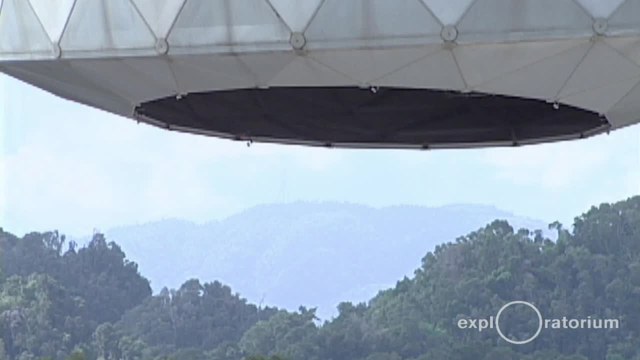 what kind of signal it is. Is it AM, FM, Is it pulsing? So it's very complex And that's So. we have a lot of different things. we want to go through and look at our data in a lot of different ways. 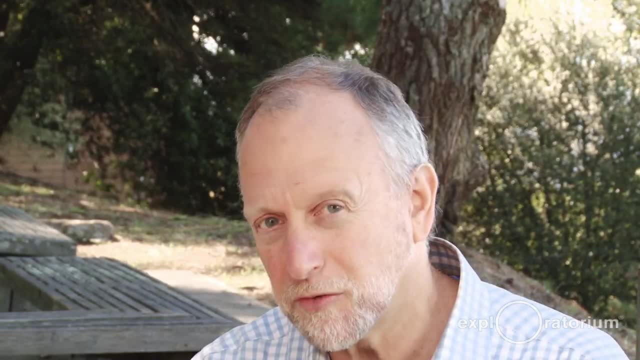 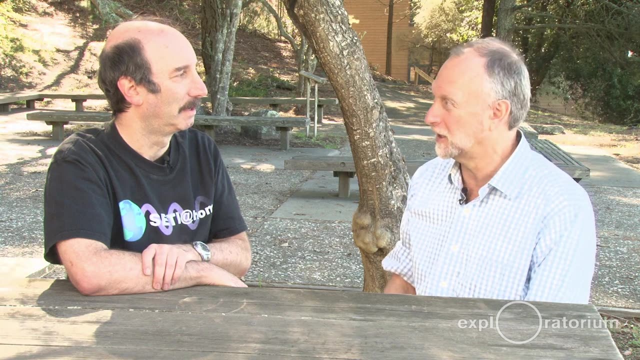 and that takes a huge amount of computing power. So what we do is we record the data at the telescope and then we send it out to the volunteers all around the world to help us analyze the data, And that's a program that you have called SETI at Home. 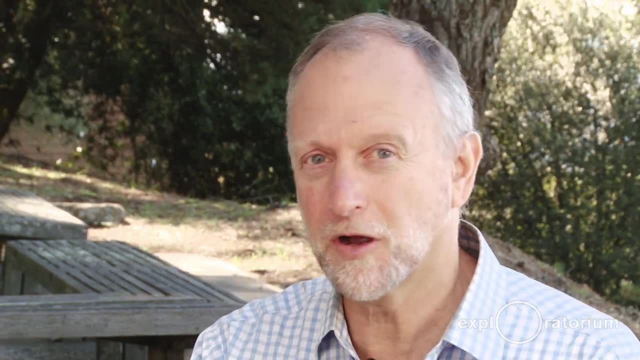 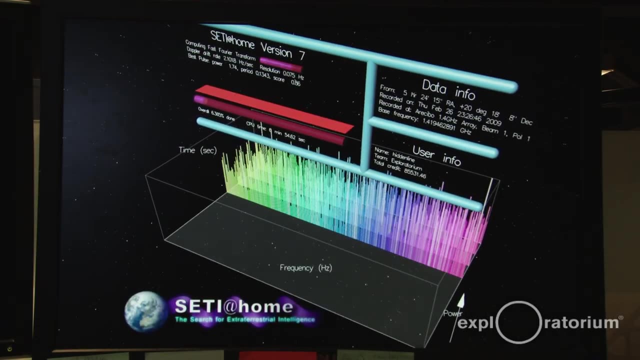 Right. It's a free program you can download. You go just Google SETI S-E-T-I and you can find the SETI at Home website. You install it on your computer and then it behaves like any other kind of screensaver. 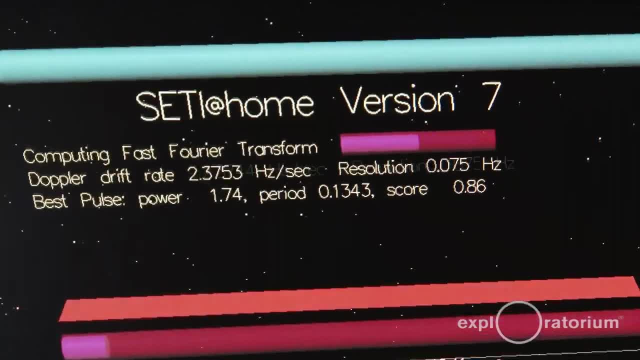 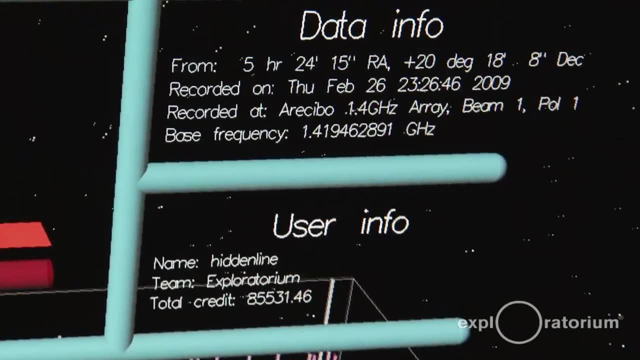 It pops up when you go out for a cup of coffee. But instead of just putting pretty pictures on your screen, it's actually going through the data, looking for that faint murmur of an extraterrestrial civilization. And your name is attached to the data. 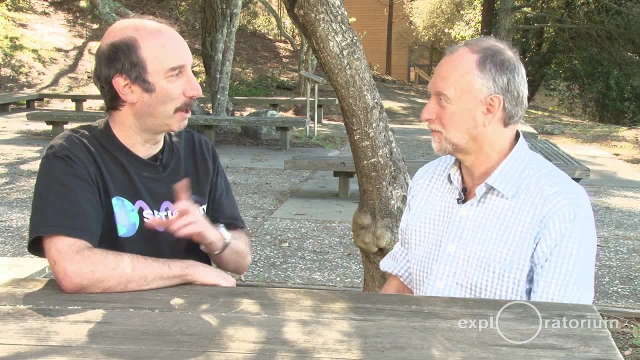 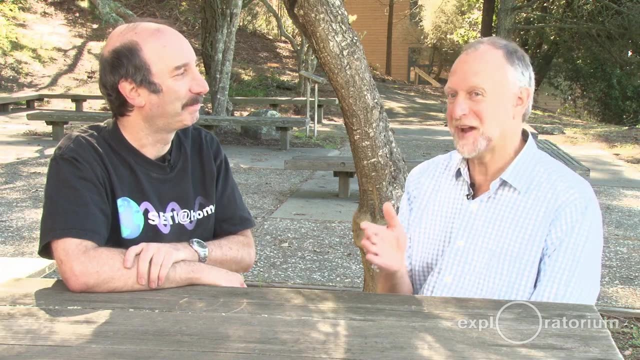 So if you're the lucky one that finds ET, you get the Nobel Prize Along with you, With me and maybe 8 million other people. Tell us a little bit about that SETI at Home receiver you have at Arecibo Right. So we just got back from the telescope where we installed this new instrument. 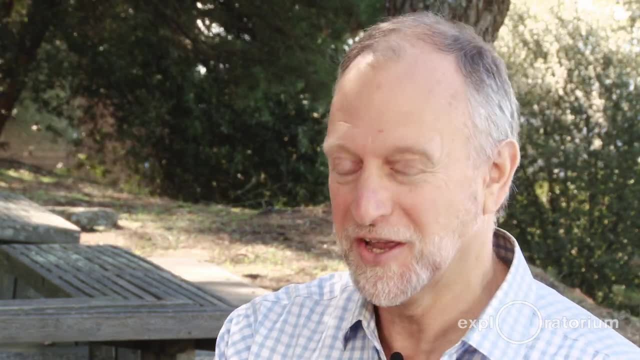 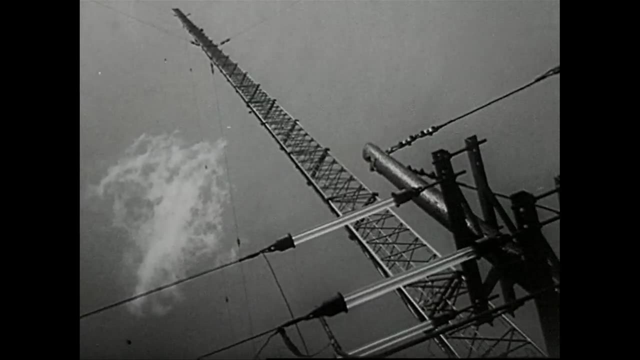 that can listen to 5 billion channels simultaneously. So the name is SETI at Home. The name of the game is to listen to as many channels as you can, because we don't know what channel ET might be broadcasting on. You don't want to do it one at a time like a police scanner. 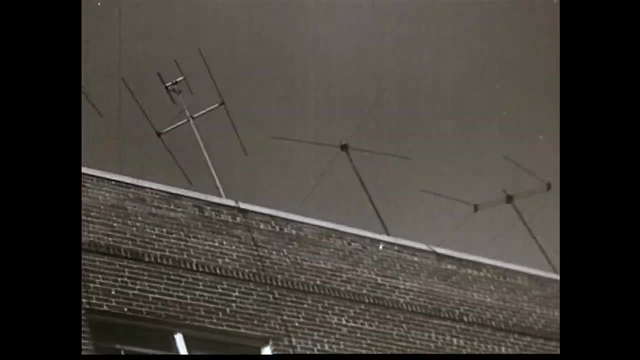 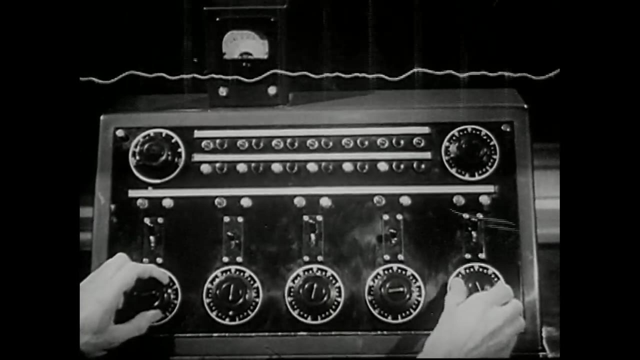 Listen here, then here, then here then here, Kind of step across the band. You want to listen to all the channels. It's like having 5 billion radios, each one tuned to a different frequency, each one listening. We're just trying to figure out if there's something strong there. 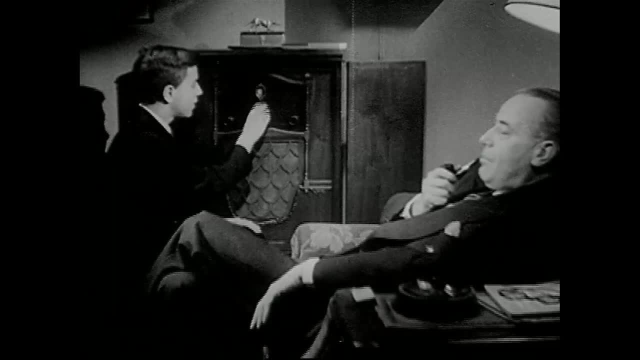 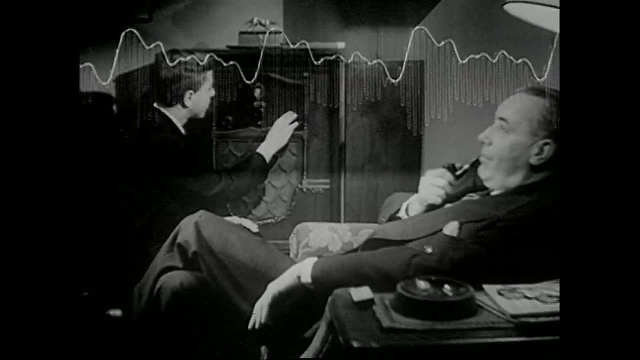 So it's like looking at the signal strength meter and seeing if it peaks up at one of those frequencies. That's what gets our attention. Then we'll go back and check it out and see if it's something really exciting. So we're trying to look at new frequency bands. 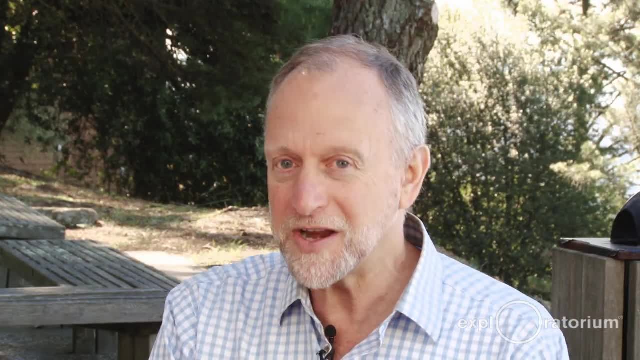 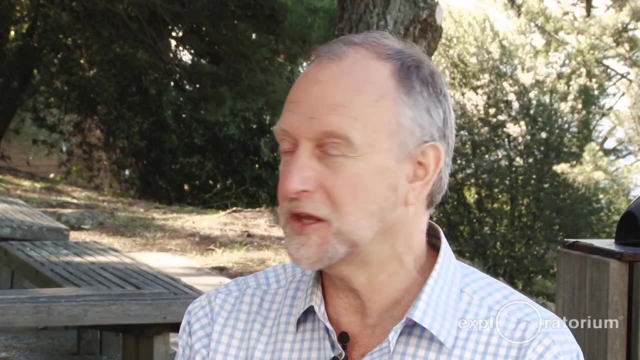 Every year we try to launch a new SETI program. We're looking at radio frequencies, now these super low frequencies. We're doing work at visible looking for laser signals, and we're also just starting off something in the infrared: looking for infrared laser signals. 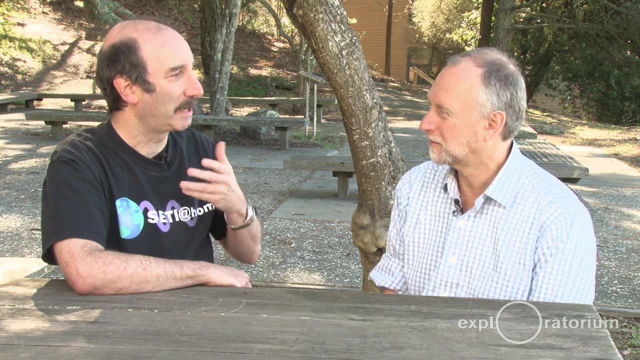 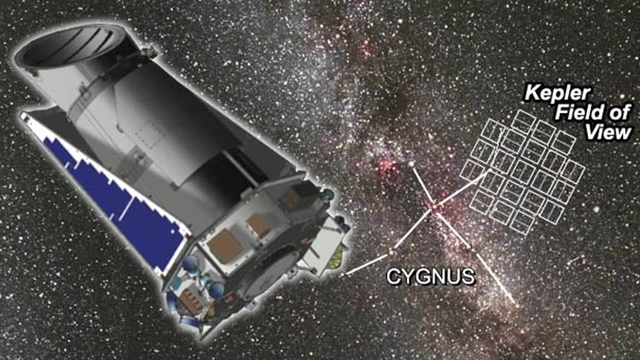 Recently we've had a lot of interesting scientific results given to us from the Kepler mission, which has discovered thousands of planets going around other stars, and that must make you feel really good. This is really exciting. You extrapolate from the few thousand planets that they found. 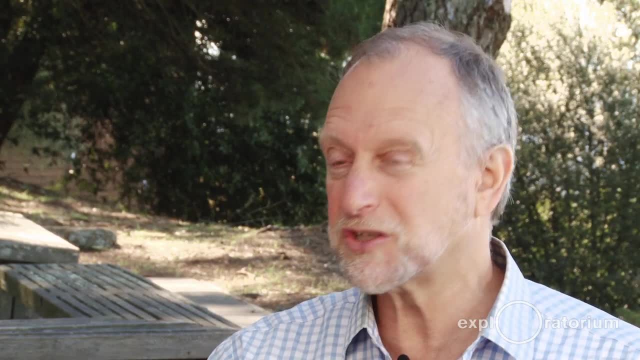 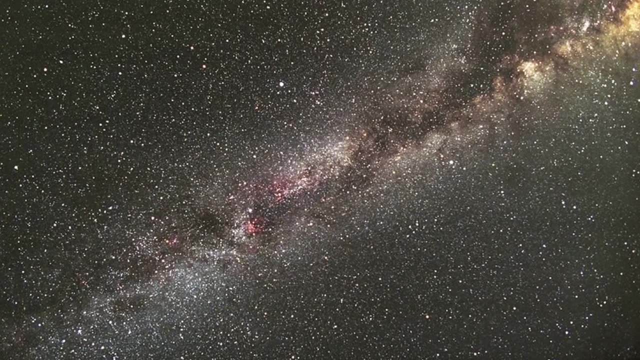 by the little patch in the sky that they looked at. you extrapolate. it looks like there's a trillion planets in the Milky Way galaxy. A trillion planets- that's five times more planets than there are stars. So there's lots of planets out there, and some of them that they found are like the Earth. 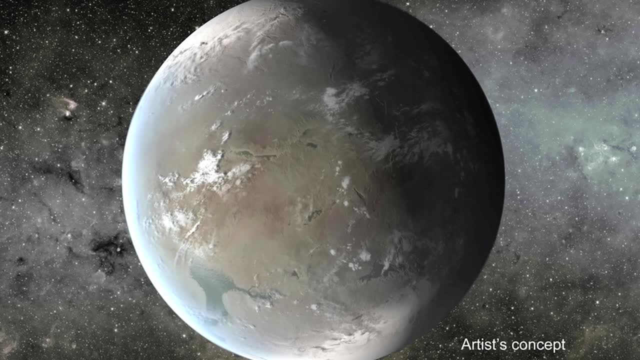 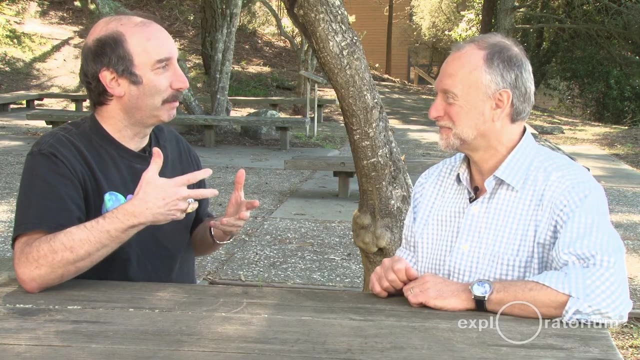 They're little dinky things and they're probably rocky, and a lot of them have liquid water. So we think that there are lots of places for life in the universe. So, Dan, there's been a history about SETI. We're not the first ones to think about it.